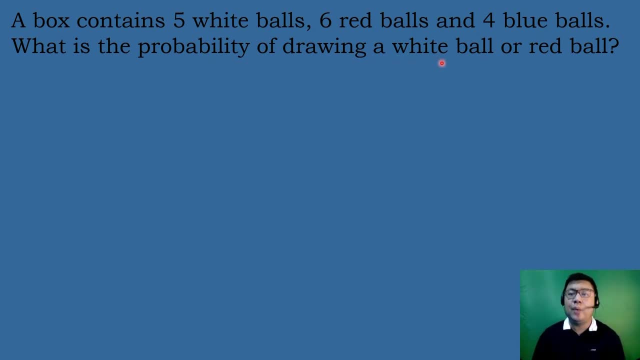 What is the probability of drawing a white ball or a red ball? Let's identify first the given. Event A, which is getting a white ball, is equal to five, because there are five white balls. Event B, which is getting a red ball. 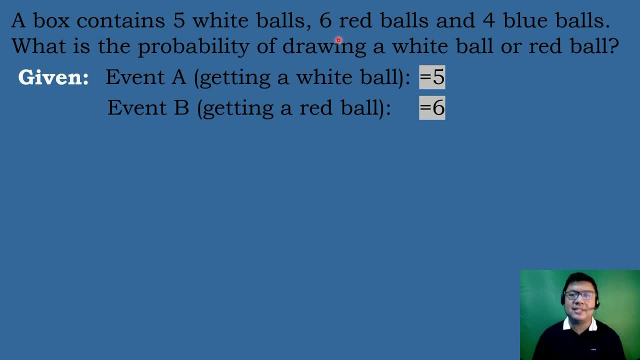 is equal to six because there are six red balls. And event C, which is getting a blue ball, is equal to four because there are four blue balls. After that, we will be identifying the total number of sample space, which is. we can solve it by adding the three events. 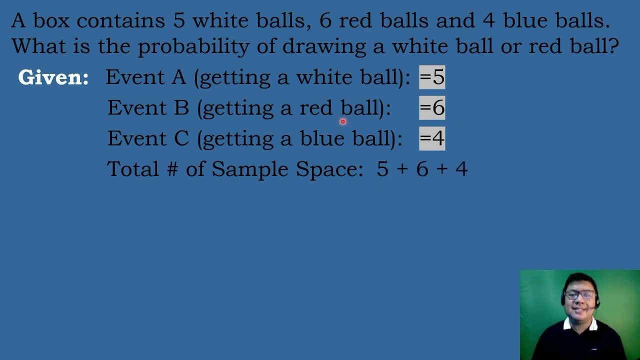 So we have five white balls, six red balls and four blue balls. So adding these numbers we will get 15.. So this is the total number of sample space. After that we will be identifying if this is an example of union or intersection of events. 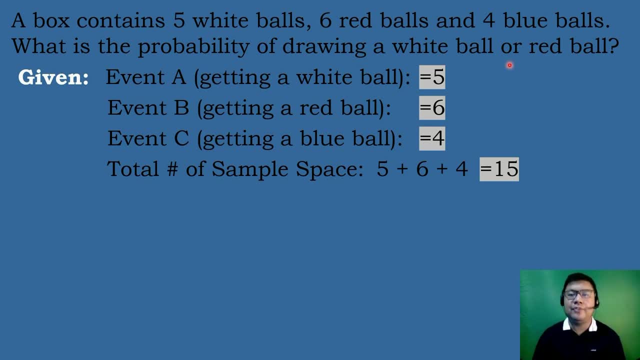 Obviously, this is an example of probability of union of events. because there is a word OR in between the white ball and the red ball, We will be using the probability of union of two events. Probability of A union B is equal to the probability of A plus the probability of B minus the probability of A intersection of B. 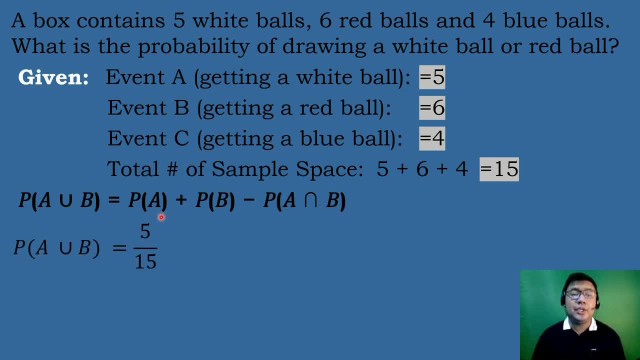 Probability of A union B is equal to the probability of A. So we have five event outcomes all over 15 total number of sample space, plus the probability of B, which is equal to 6. event B: all over the total number of sample space, which is equal to 15, minus the probability of a intersection. 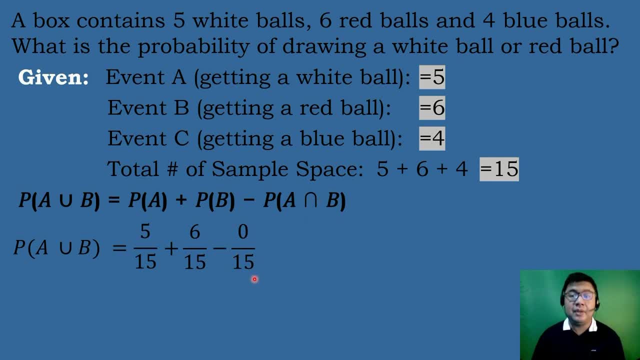 B, which is equal to 0 over 15, because there is no intersection between the white ball and the red ball. so 0 event outcomes all over the total number of sample space, which is equal to 15. and then we will be simplifying this one. 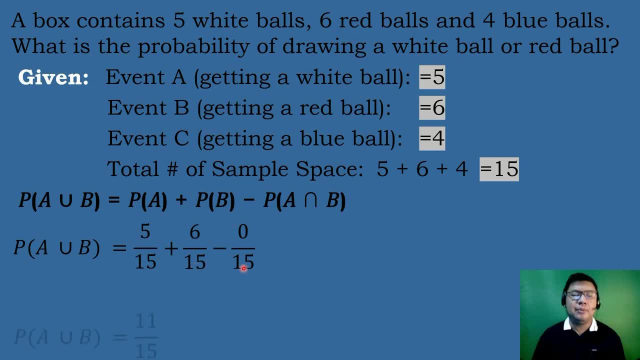 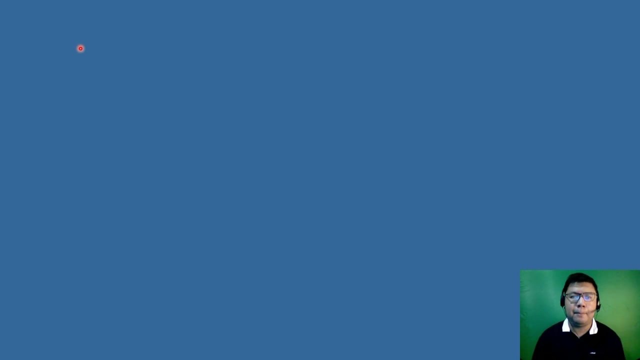 since this is an example of similar fraction, we will just copy the denominator 15 and then add the numerator 5 plus 6 will be equal to 11. therefore, the probability of getting a white ball or getting a red ball is equal to 11 over 15. let's have our second example. 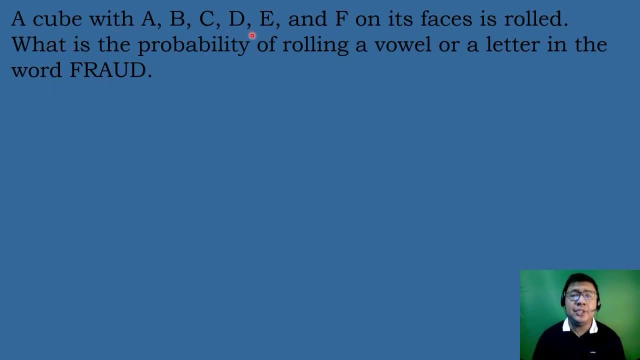 let's have our second example. let's have our second example. a cube with letters A, B, C, D, E and F on its pieces is rolled. what is the probability of rolling a ball or a letter in the word prod? let's identify first the given. so event outcomes of a which is rolling a bowel is equal to the. 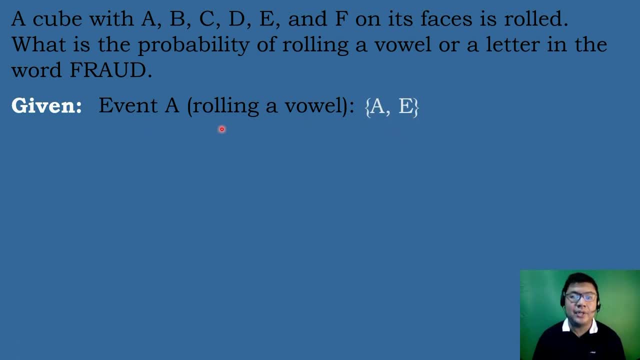 letters A and E, because these are the bowels that can be found from the letters A, B, C, D, E and F, and that is equal to 2. after that, event outcomes for event B: rolling a letter in the word prod is equal to the letters A, D and F. letter A is found on the word. 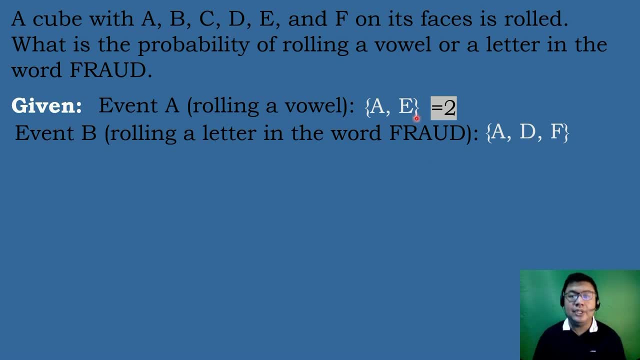 prod. same goes with letter D and letter F. so this are the three letters. so we have event B, which is equal to 3, and then for event A, intersection B, what are the letters that occurred in both events? we have the letter A, so we have A here. 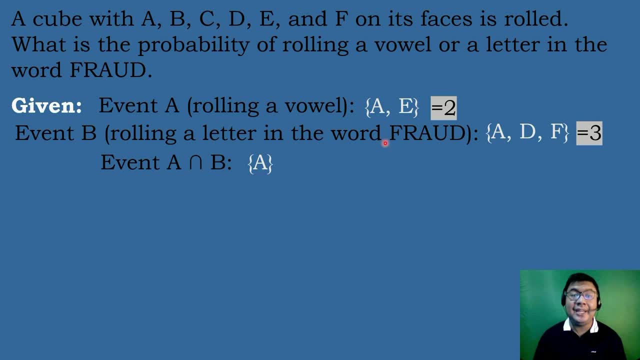 for event A and then another A here for event B. so A occurred on both events. so therefore the intersection of A and B is the letter A, so it is equal to 1. so that's it for today's lesson. Thank you for watching. See you next time. 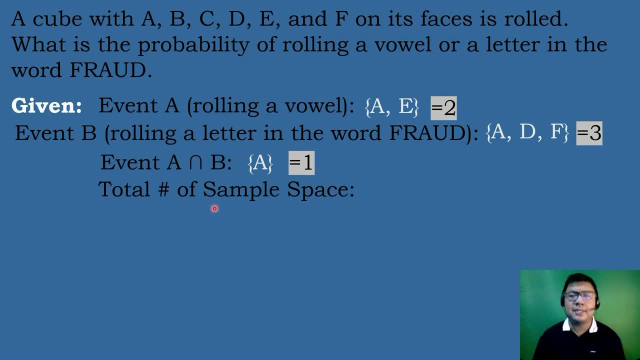 and then after that let's identify the total number of sample space. so the total number of sample space is equal to 6, because there are 6 letters on a cube, and then we will be identifying if this is an example of union or intersection of events. and obviously this is an example of union of two events because 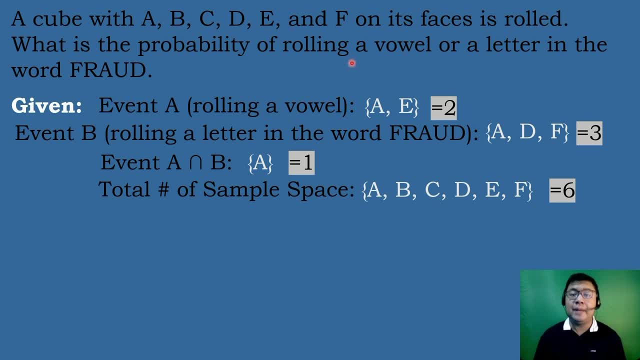 there is a word or in between rolling a vowel and a letter. in the word prod, we will be using the formula for union of two events. probability of a union B is equal to the probability of a plus probability of B minus probability of a intersection B. after that we will bring down: the probability of a union B equals the. 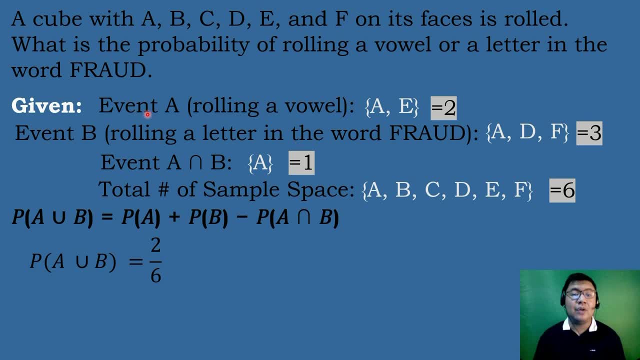 probability of a, so event outcomes of a rolling a vowel is equal to 2. all over, the total number of sample space is equal to 6 plus the, Thus the probability of B, so event outcomes of B is equal to 3,. all over, the total number of sample space is equal to 6, minus the probability of A intersection B, so event outcomes of A intersection B is equal to 1, and then the total number of sample space is equal to 6.. 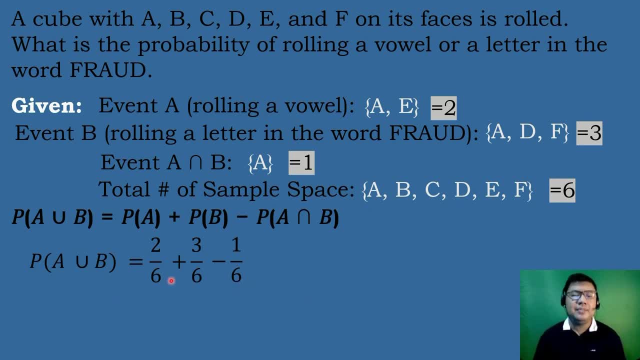 Since this is an example of similar fraction, we will just copy the denominator and then add the numerator. So we have 2 plus 3 is 5, minus 1 is equal to 4.. 4 over 6- lowest term- is equal to 2 thirds. 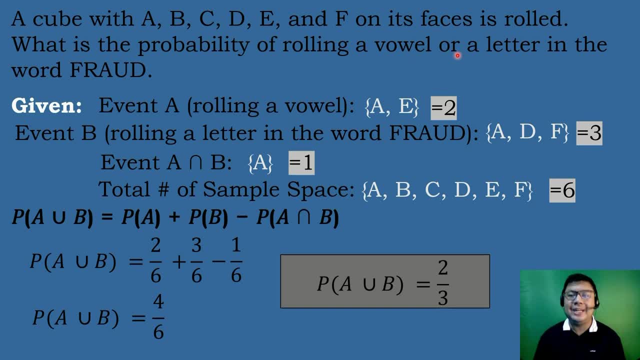 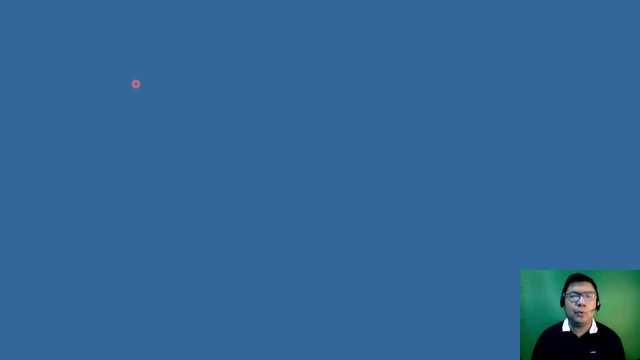 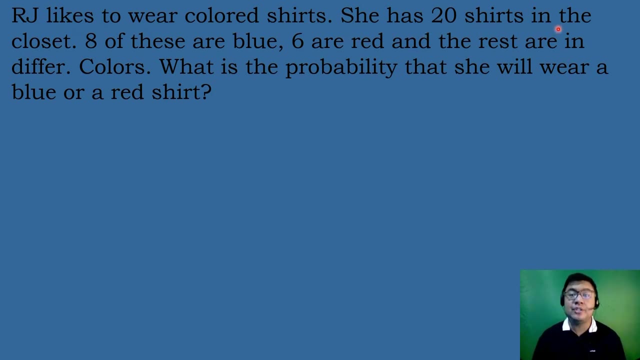 Therefore, the probability of rolling a vowel or a letter in the word prod is equal to 2 thirds. Let's have our next example. RJ likes to wear colored shirts. She has 20 shirts in the closet. 8 of these are blue, 6 are red and the rest are in different colors. 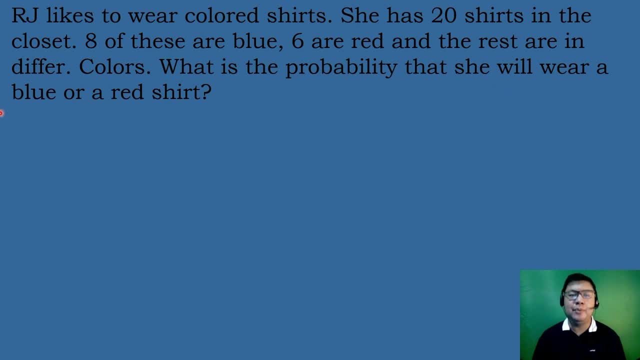 What is the probability that she will wear a blue or a red shirt? Let's identify first the given. So event outcomes of A, which is getting a blue shirt, is equal to 8.. Event outcomes of B, which is getting a red shirt, is equal to 6.. 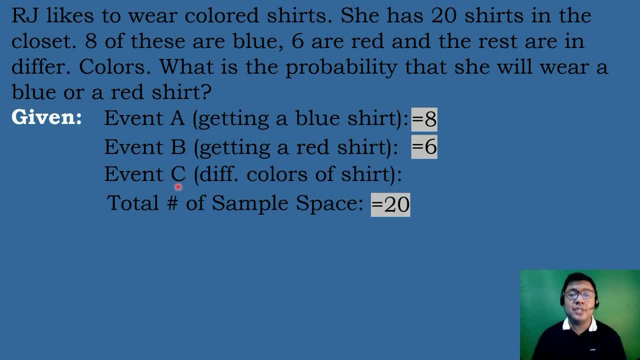 And then after that event outcomes of C, which is different colors of shirt, is equal to 20, the total number of shirts minus the quantity of the sum of the blue shirts and the red shirts, So we have 8 plus 6.. 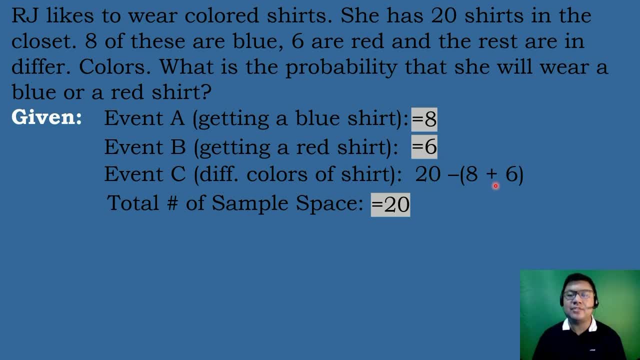 8 plus 6 is equal to 14, then 20 minus 14 will be equal to 6.. So therefore, event outcomes of C, which is getting a different colors of shirts, is equal to 6.. And then the total number of sample space is equal to 20,, which is already given. 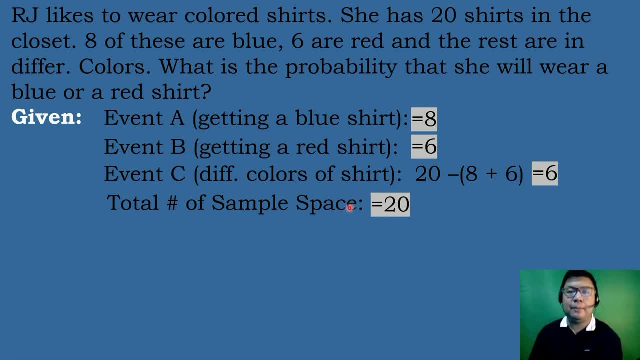 We will be identifying if this is an example of union or intersection of two events. So there is a word or intersection In between the blue shirt and the red shirt. therefore, this is an example of union of two events. We will be using the formula of probability of A union B is equal to the probability of A plus probability of B minus probability of A intersection B. 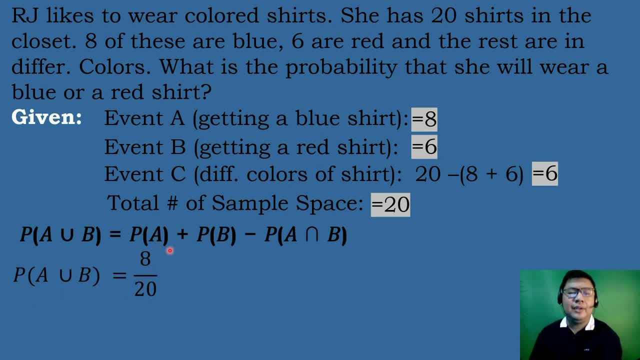 And for the probability of A, we have event outcomes of A, which is equal to 8.. All over, The total number of sample space, which is equal to 20.. Plus the probability of B, so event outcomes of B getting a red shirt is equal to 6.. 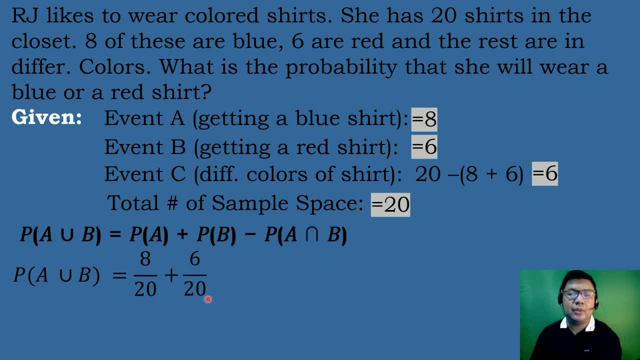 All over the total number of sample space, which is equal to 20.. Minus the probability of A intersection B, so the total number of sample space is equal to 20.. And A intersection B: the intersection of A and B is equal to 20.. 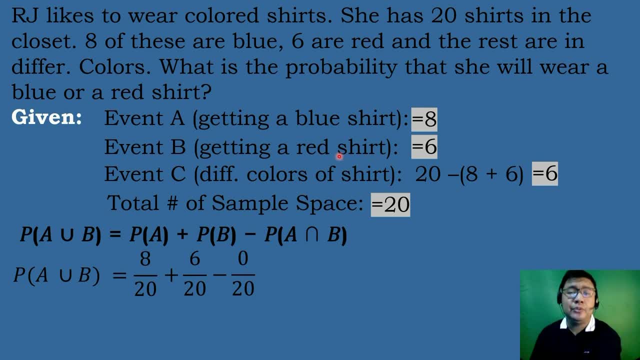 It's equal to 0, because she cannot wear a blue shirt and a red shirt at the same time. So this is equal to 0.. And then we will be simplifying this one. Similar proctions: Copy the denominator and then add and subtract the numerator. 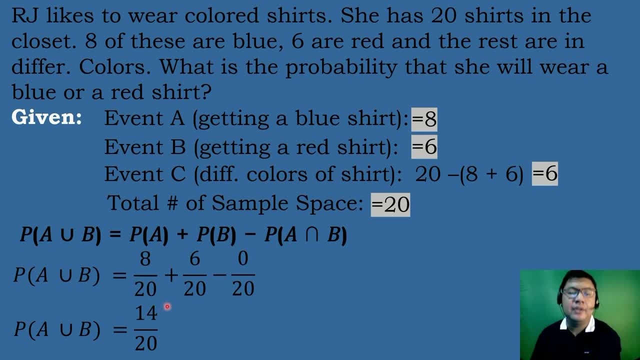 So 8 plus 6 is equal to 14 minus 0, 14.. So we have 14 over 20 and lowest term is equal to 7 over 10.. Therefore, the probability that she will wear A blue shirt. 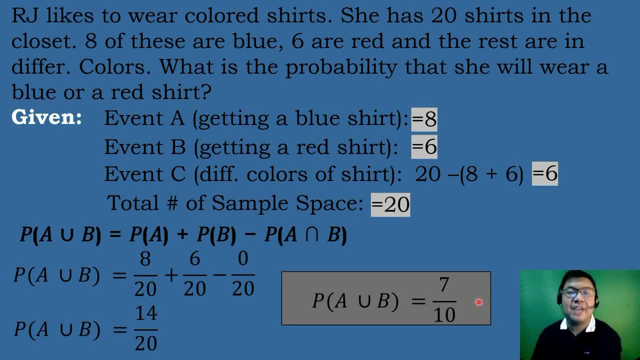 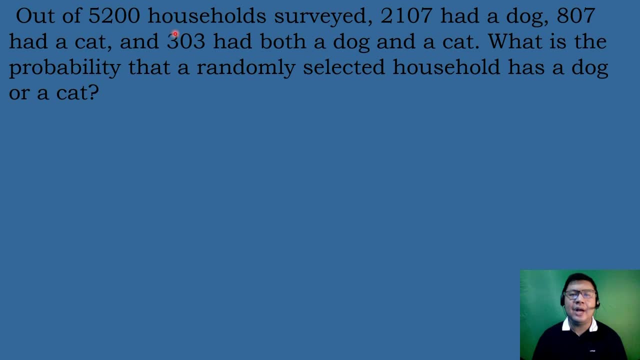 blue or a red shirt is equal to 7 over 10.. let's have another example: out of 5200 households surveyed, 2107 had a dog, 807 had a cat and 303 had bought a dog and a cat. what is the probability? 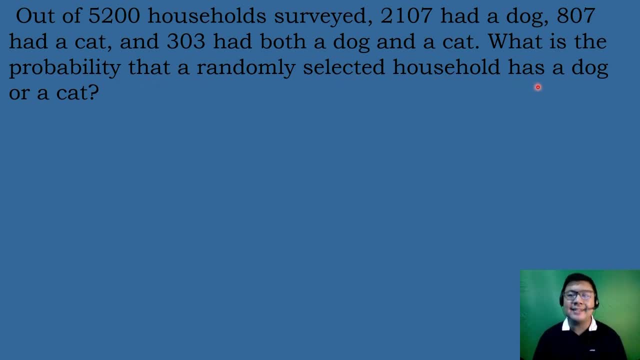 that a randomly selected household has a dog or a cat. let's identify first the given. so we have event outcomes of a- the household with a dog is equal to 2107. and then we have event outcomes of b- the household which has a cut is equal to 807. and then the intersection of a and b. 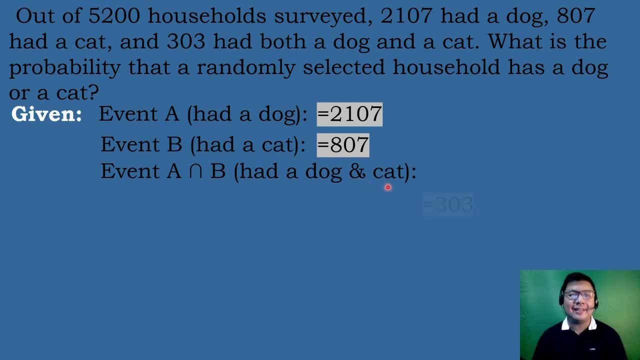 the household with a dog and a cat is equal to 303, and then the total number of sample space is already given in the problem, which is equal to 5200. we will be identifying if this one is union or intersection of events. and since there is a word or in between dog and cat, so this is an example of union of two. 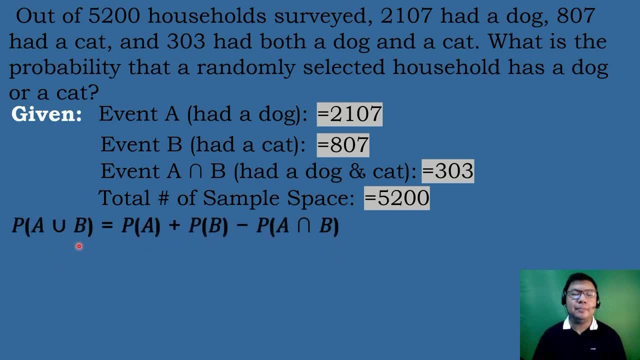 events. so we have: probability of a union b is equal to the probability of a, plus probability of b, minus probability of a intersection b, and then after that bring down probability of a union b equals probability of a, so we have event outcomes of event a, which is equal to 2107. 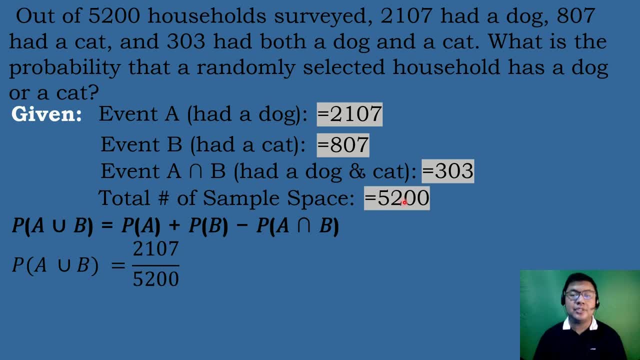 all over the total number of sample space, which is equal to 5200, plus the probability of b. event outcomes of b is equal to 807. all over the total number of sample space, which is equal to 5200, minus the probability of a intersection. b is equal to the event outcomes. 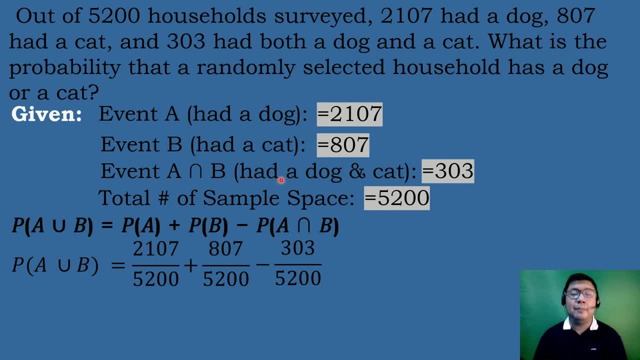 of a, intersection b, the household with both dog and cat, which is equal to 303. all over, the total number of sample space is equal to 5200. and since this is an example of similar fraction, just copy the denominator and then add and subtract the numerator 2107 plus 807 minus 303. 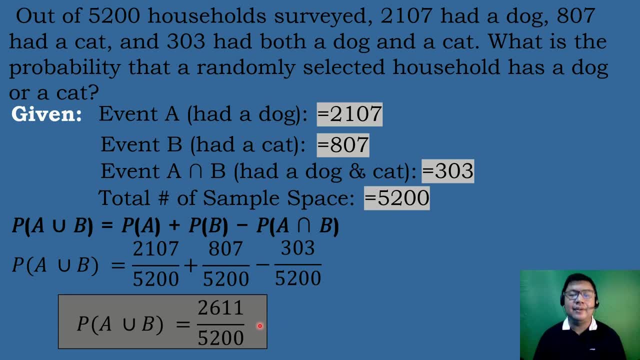 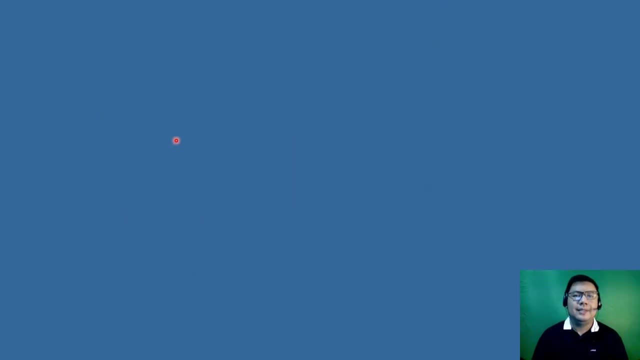 is equal to 2611.. therefore, the probability of randomly selecting a household which has a dog or a cat is equal from 120 to 150, then b, that is 202 taking the denominator and subtracting the numerator 2611 over 5200.. Let's have our last example: A die is rolled. What is the probability of? 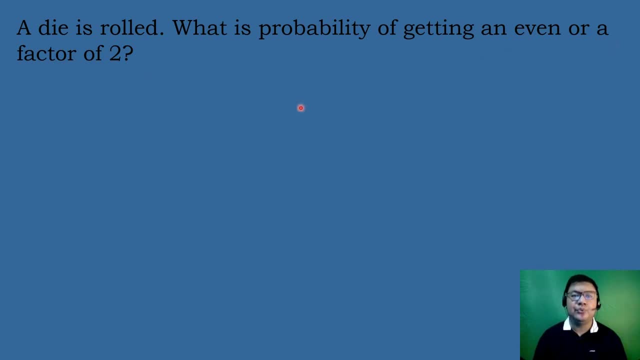 getting an even number or a factor of 2? Let's identify the given Event outcomes of A, which is rolling, and even numbers are the numbers 2,, 4, and 6.. So the event outcomes of A is equal to 3.. 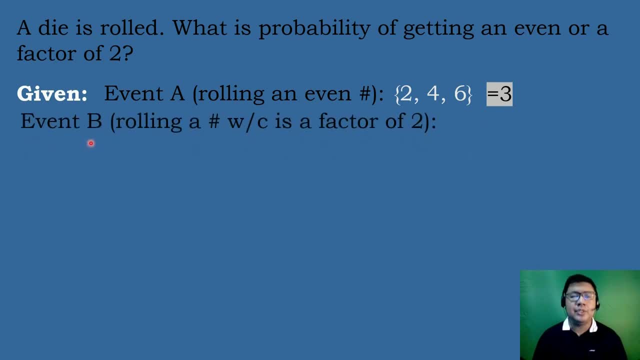 And then event outcomes of B, which is rolling a number, which is a factor of 2.. What are the factors of 2?? So that is also 2,, 4, and 6, which is also equal to 3.. And then event A intersection B. 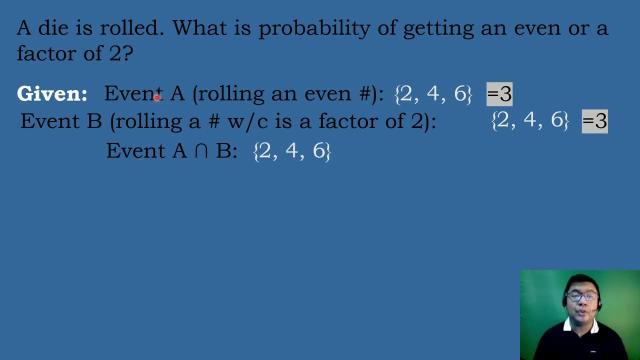 So these are the numbers that occurred on both events, Event A and event B. So we have 2,, 4, and 6. So all these numbers occurred on both events. So event A, intersection B is also equal to 3.. And then the total number of sample space. So a die is rolled, So there are 6 numbers in. 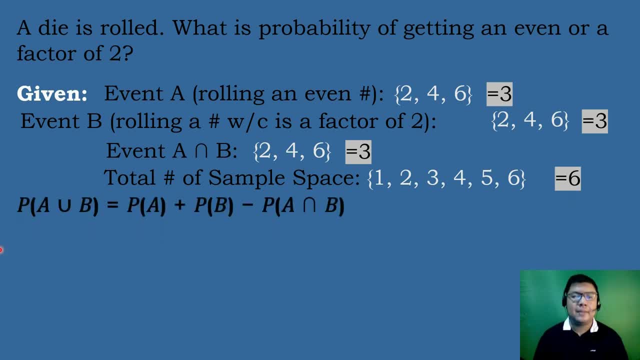 a die, So that is equal to 6.. And then after that we'll be using the formula: Probability of A union B is equal to the probability of event A plus probability of event B minus probability of event B, So that is equal to 6.. And then after that we'll be using the formula. 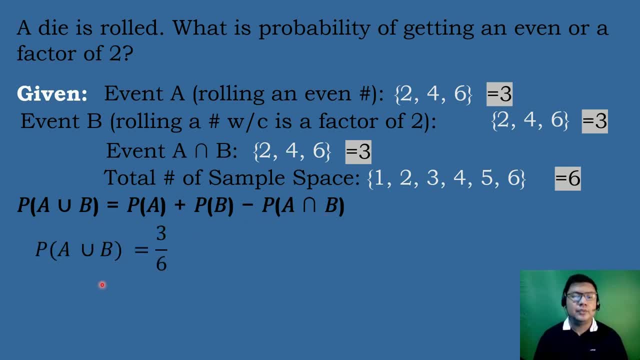 Probability of A intersection B. So we have: probability of A union B equals probability of A. Event outcomes of A is equal to 3.. All over, the total number of sample space is equal to 6, plus the probability of B is equal to 3.. And then the total number of sample space is equal to 6.